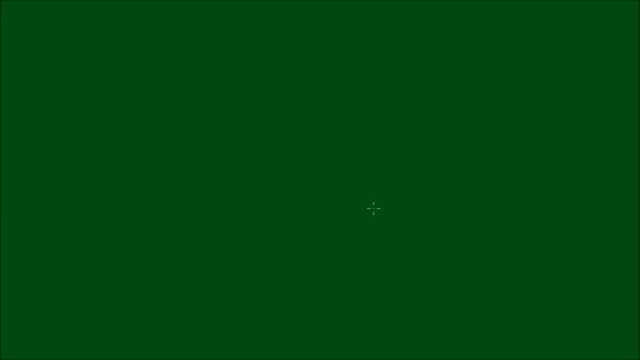 In this video we are going to explore the roots of a fourth-order polynomial to its coefficients. So let's start off with an arbitrary fourth-order polynomial: ax to the fourth, plus bx to the third, power plus cx. squared plus dx plus e is equal to zero, And I'm going. 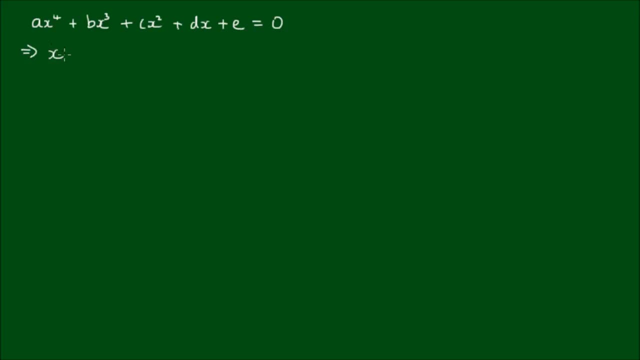 to rewrite this equation by dividing through by a, so I get x to the fourth, plus b on a, x cubed, plus c on a, x squared, plus d on a, x plus e on a is equal to zero. And let's suppose that the constants that satisfy this equation are alpha, beta, gamma and theta. 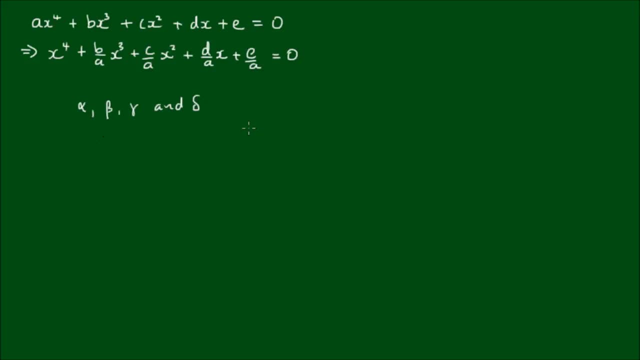 So alpha, beta, gamma and delta are the roots or zeros. This then means I can write this equation as the multiplication of x minus alpha by x minus beta, x minus gamma and x minus delta, And if I then proceeded to expand all of these terms out, I would get the following relationships: 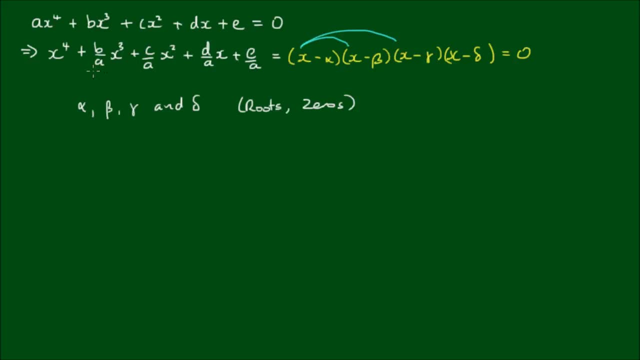 between these roots and the coefficients. So the sum of all of the roots, which I'll write shorthand as the sum of alpha, which is alpha plus beta plus gamma plus delta, is equal to the negative of b on a, So the negative of the x cubed coefficient. Then the sum of the paired combinations of the roots which 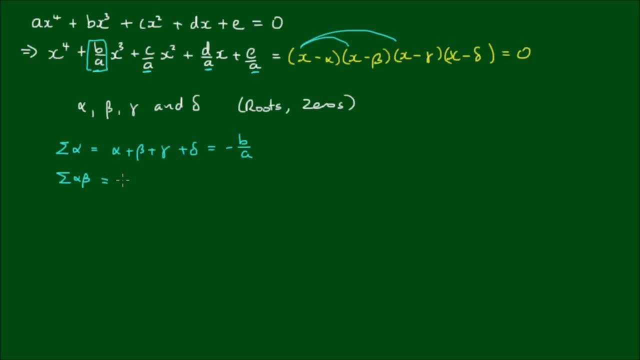 I'll write shorthand as the sum of alpha beta, and this is equal to alpha beta plus alpha gamma plus alpha delta plus beta gamma plus beta delta plus gamma delta is equal to c on a. So the positive of the x squared coefficient or the quadratic coefficient, Then the sum. 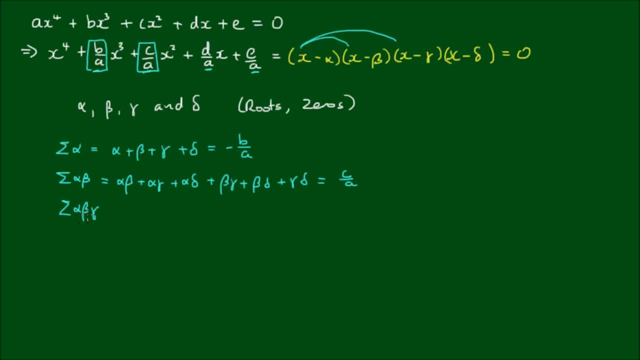 of the triple combinations of the roots, the sum of alpha by beta by gamma, which is alpha by beta by gamma plus alpha beta delta plus alpha gamma delta plus beta gamma delta, is equal to negative d on a, So the negative of the x coefficient or the linear coefficient. 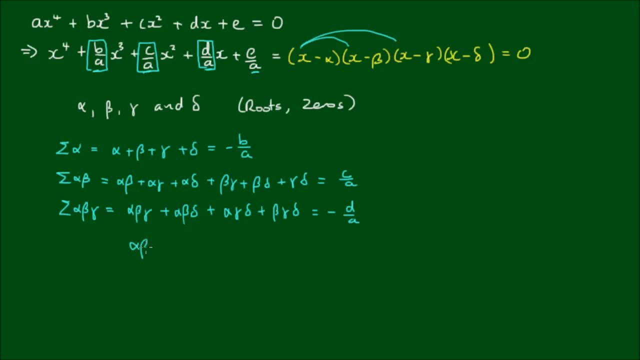 And then the multiplication of all of the roots, so alpha by beta, by gamma, by delta, is equal to e on a, So equal to the free term. So these are all of the relationships between the coefficients of the polynomial, So the polynomial and the four roots of the polynomial. And note that, since we have a fourth order, 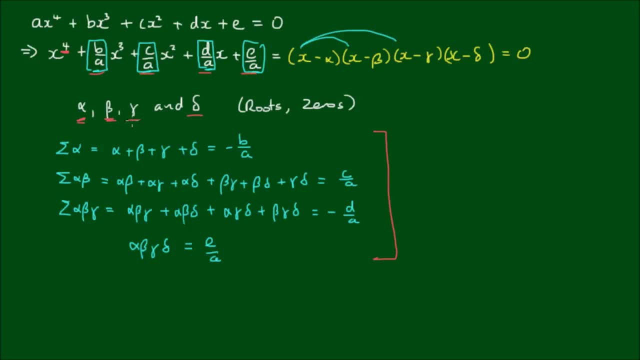 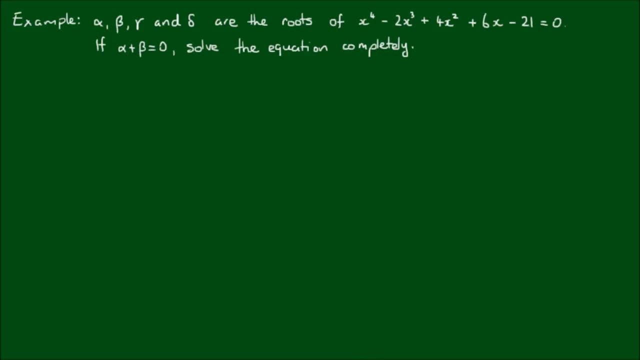 polynomial, normally we would expect to get four roots. So, knowing this, let's do an example. Okay so alpha, beta, gamma and delta are the roots of x to the fourth. minus 2x cubed, plus 4x squared plus 6x minus 21 equals 0.. If alpha plus beta equals 0, solve the equation. 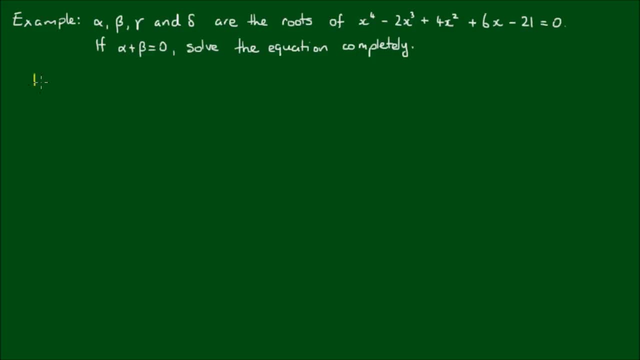 completely. So first of all, let's write down all of the relationships. So we have: alpha plus beta plus gamma plus delta is equal to positive 2, because it is negative of the x cubed coefficient. Second, we have alpha beta plus alpha gamma plus alpha delta plus. 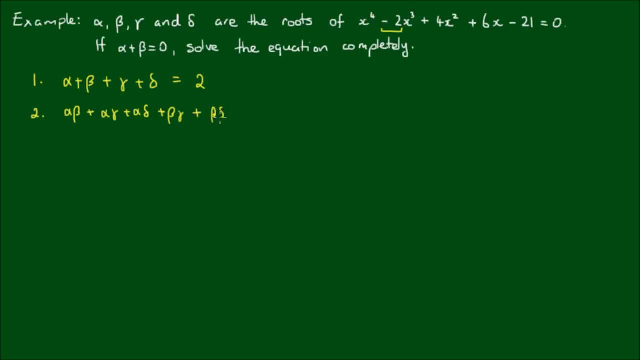 beta gamma plus beta 2x squared plus 6x minus 2x squared plus 6x minus 2x squared plus 6x plus 0x plus x squared plus delta plus gamma delta is equal to 4, which is the x squared. 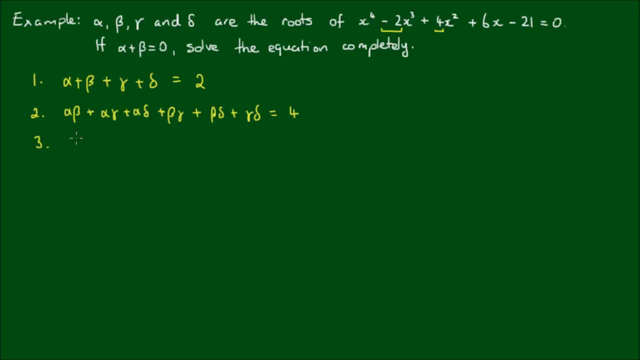 coefficient. Thirdly, we have alpha beta gamma plus alpha beta delta plus alpha gamma delta plus beta gamma delta is equal to 4.. So this is the x squared coefficient. negative 6, so negative of the linear coefficient. 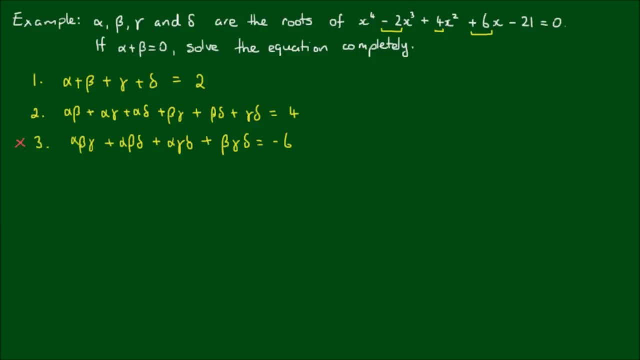 But, as you'll find out, we won't actually need this relationship. And fourthly, we have alpha times, beta times, gamma times. delta is equal to negative 21.. And I'm going to circle 1, 2 and 4 to call these relationships equation 1, equation 2 and equation 4.. 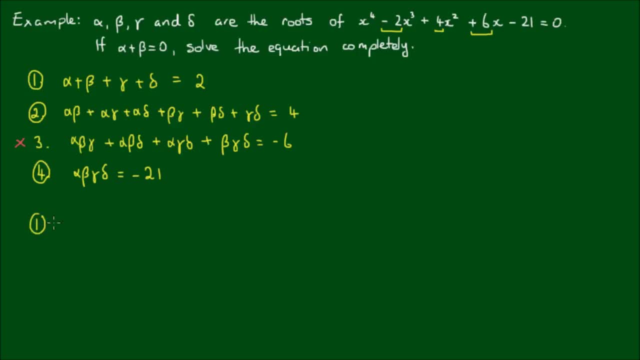 So if we take equation 1, we have alpha plus beta, plus gamma plus delta is equal to 2.. Well, since alpha plus beta equals 0, we have gamma plus delta is equal to 2.. And now let's take equation 2.. 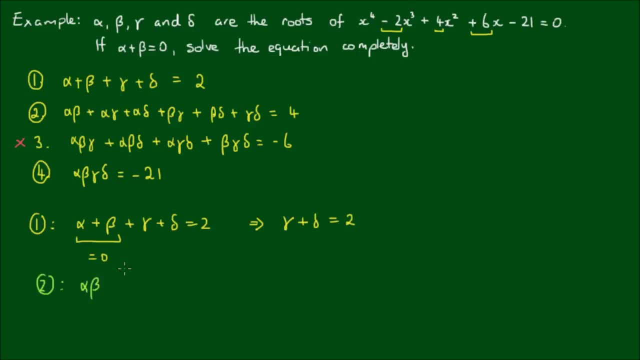 So firstly, we have alpha beta, But I can factor out an alpha in the second and third terms. So I have alpha outside of gamma plus delta And I can factor a beta out of the fourth and fifth terms to get beta outside of gamma plus delta. 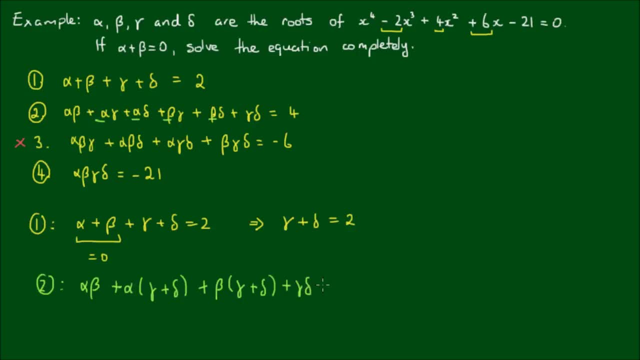 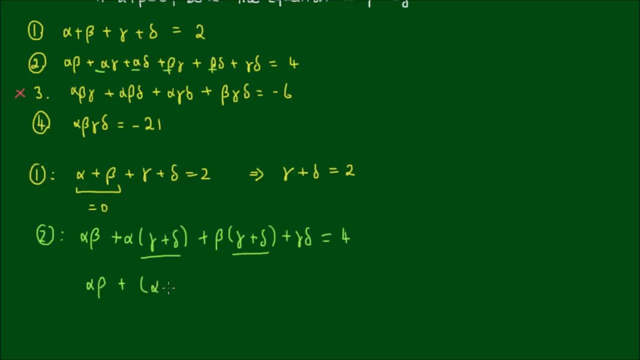 And then the final term, gamma times delta, remains, and this is equal to 4.. And note that now I can factor out gamma plus delta, So I have alpha beta plus alpha plus beta times, gamma plus delta plus gamma delta is equal to 4.. 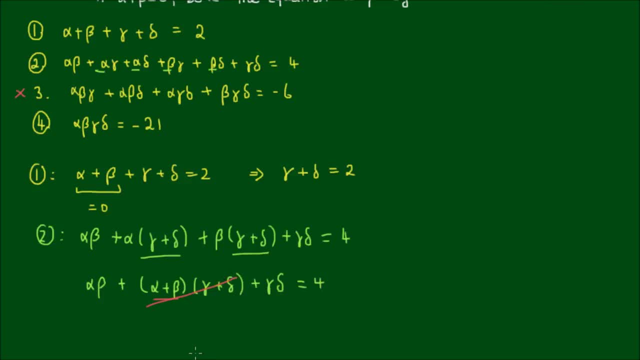 And since alpha plus beta equals 0,, this term disappears. So we have: alpha beta plus gamma delta is equal to 4.. So let me write that down: Alpha beta plus gamma delta is equal to 4.. And let me call this equation 5.. 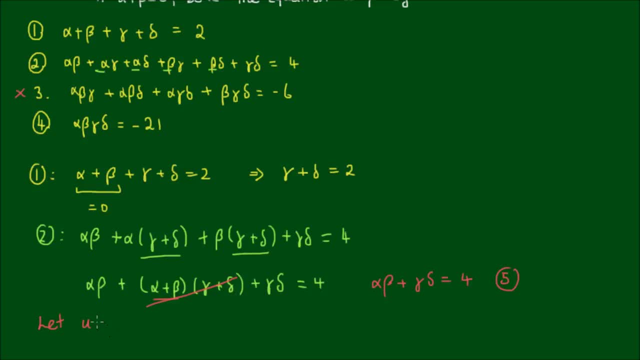 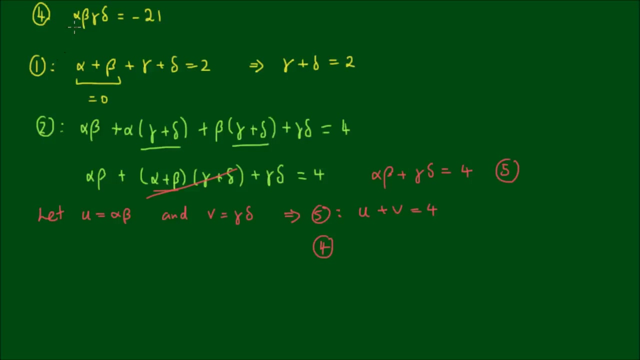 Now I'm going to let: u is equal to alpha beta, just to simplify things, And I'll also let: v equals gamma by delta. So equation 5 becomes: u plus v equals 4.. And equation 4- we have u times v is equal to negative 21.. 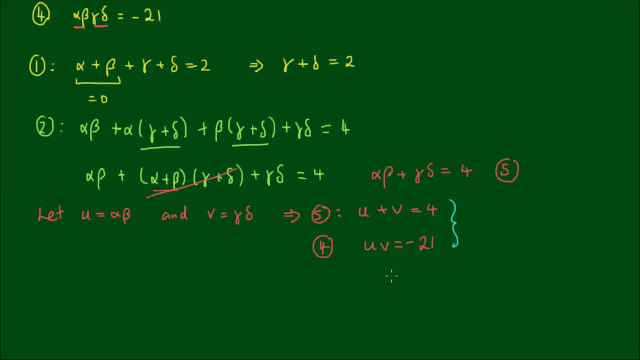 So now we can solve these equations simultaneously. So the factors of negative 21 are negative 1 and 21. And these add to give 20.. The next set of factors is negative 3 and 7. And these add to give 4.. 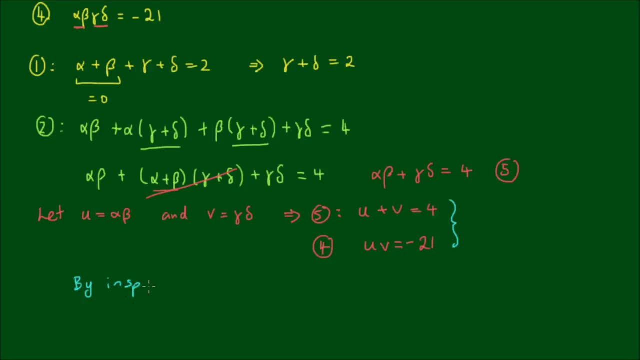 So, by inspection, u is equal to negative 3.. And v is equal to 7.. So, with u being equal to negative 3,, this implies that alpha beta is equal to negative 3.. Since we let u equals alpha beta And we also have alpha plus, beta equals 0,. 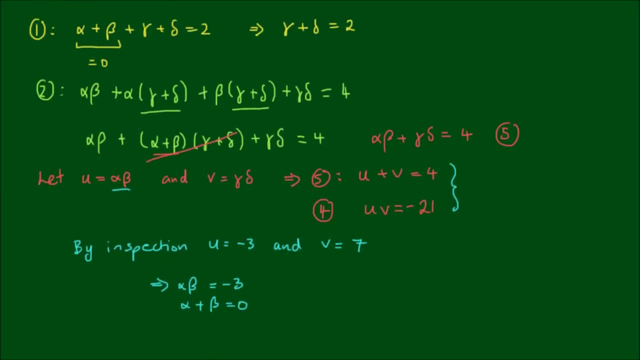 which is the initial condition that we were given. So, to satisfy this system of equations, we have the result: alpha is equal to the square root of 3. And beta is equal to the negative of the square root of 3.. And you can satisfy yourself that this result satisfies this system of equations. 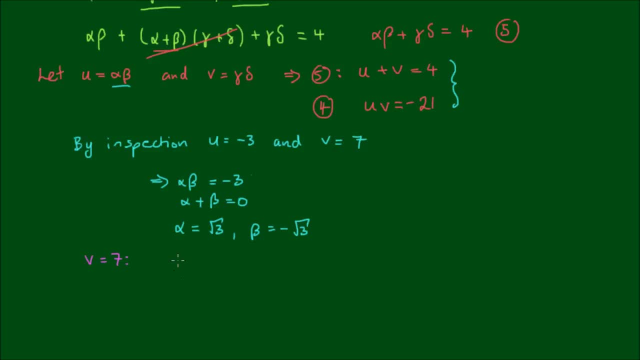 And now, with v equals 7,, we have gamma: delta is equal to 7. And gamma plus delta is equal to 2.. So I can write delta is equal to 2 minus gamma And then sub it into gamma: delta is equal to 7.. 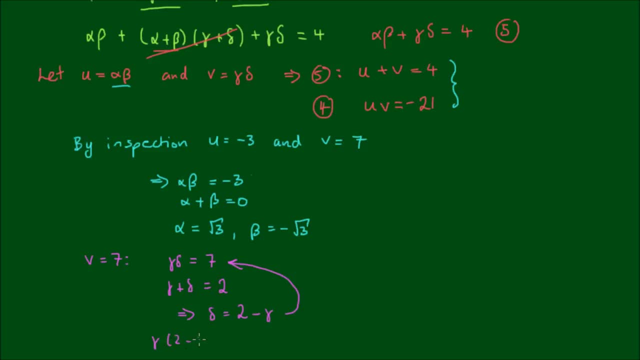 And this will leave me with gamma times 2 minus delta. So v is equal to 7.. Which expands out to the quadratic gamma squared minus 2, gamma plus 7 is equal to 0.. And if we use the quadratic formula to solve for this, 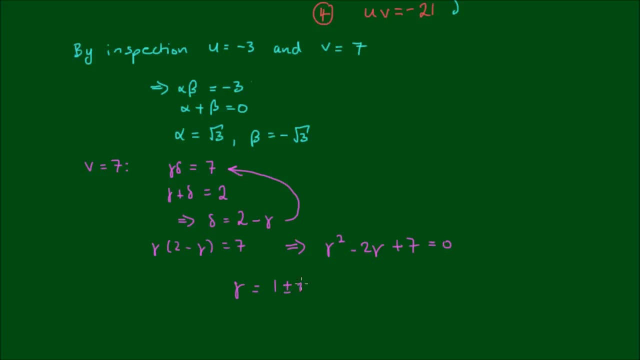 we get. gamma is equal to 1 plus or minus i times the square root of 6.. And now we don't actually have to solve for delta here, because if we substitute this result into here, we get pretty much exactly the same result.